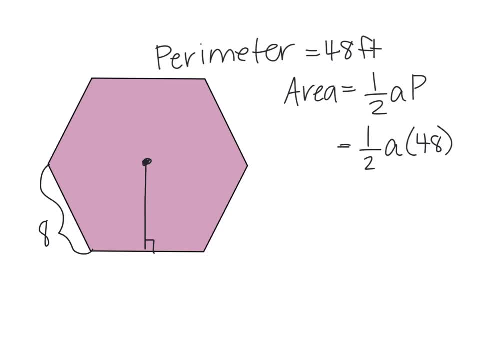 48 divided by 6 is 8.. So each side on the hexagon has a value of 8.. That means if we want to calculate our apothem, which is the distance from the center to any of the sides perpendicular, then we are going to cut that 8 in half. 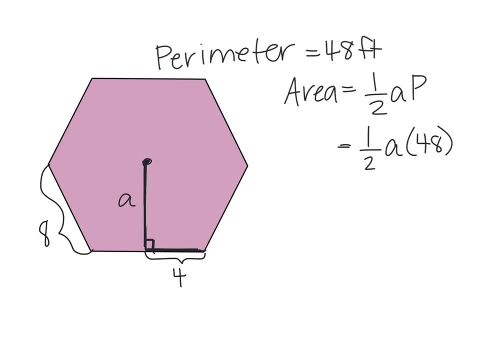 right here to get 4.. So if we have this right triangle, we want to think about what would be the angle that we want to use right here. So I know that if I were to cut this up into different equal parts for a hexagon, if we did, 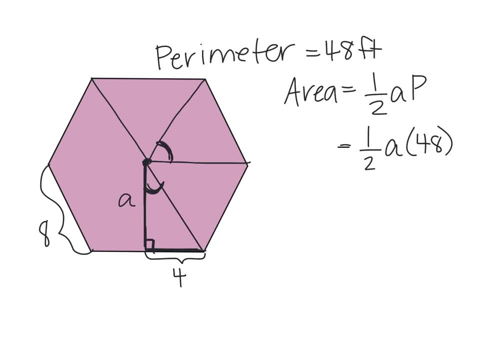 360 degrees divided by 6, that's going to be a 60 degree angle. That means, for the one that I'm looking at right here, this angle- since we bisected my side- that is going to be an angle of 30 degrees. So now we're actually looking at 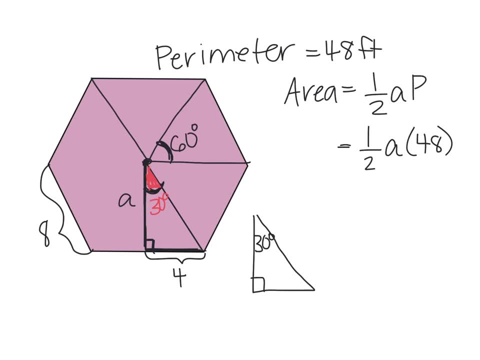 a 30,, 60,, 90 right triangle. So there's several ways you could solve this. You could use trigonometry. So SOH CAH, TOA, We have this. 4, which represents the opposite side of the 30 degree. 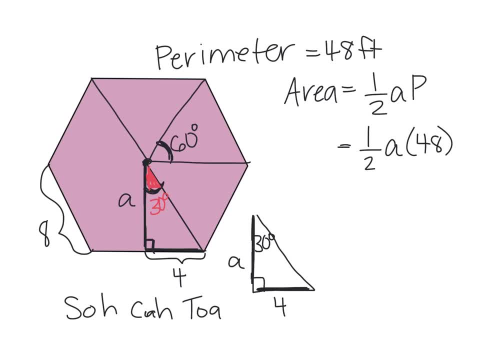 angle and we're trying to solve for the apothem, which is the adjacent side. We could use tangent of 30 degrees here to solve. Or, since we know that this is a special right triangle, I know that the side that is opposite from the 60 degree angle has to be 4. 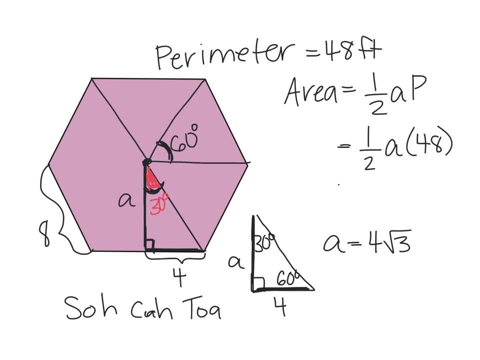 times the square root of 3.. So now I'm going to use that in my answer here and we should get a value of 2 times the square root of 3, a total area rounded since I multiplied by the square root of 3, 166.28.. If we round here, that's going to be square.